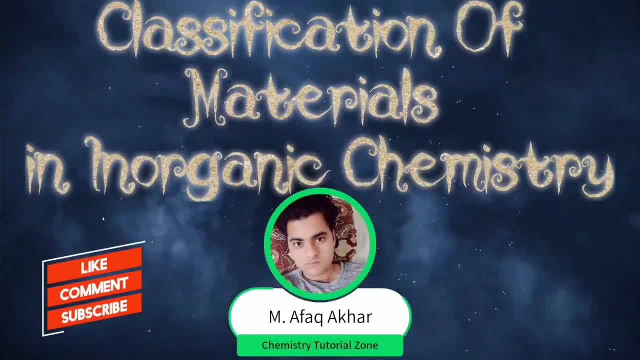 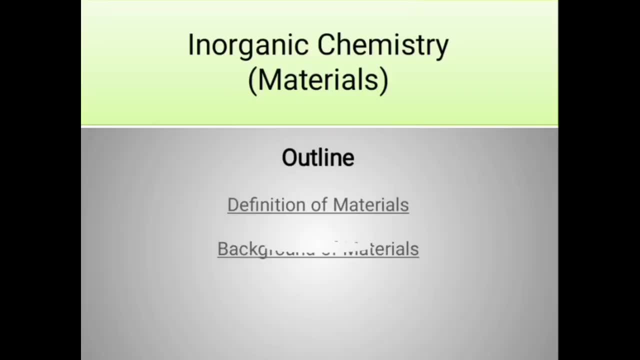 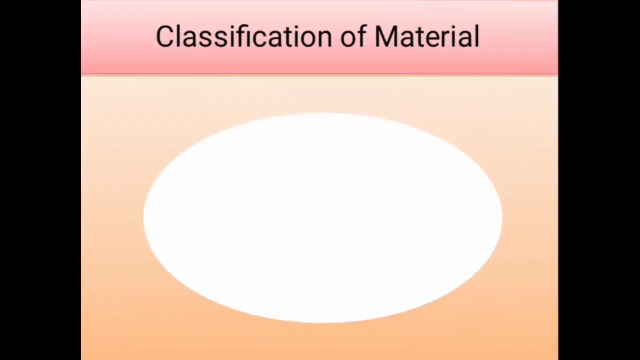 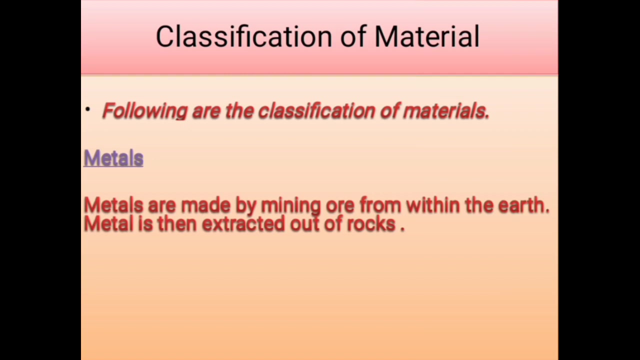 Hello students. today I will explain that. what are the classification of materials Moving or the classification of materials Number one is metals. Metals are made by mining ore from within the earth. Metal is then extracted out of rocks. Three types of metals. Number one is ferrous, which included 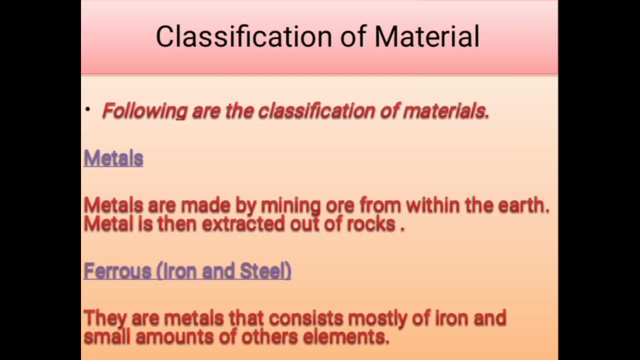 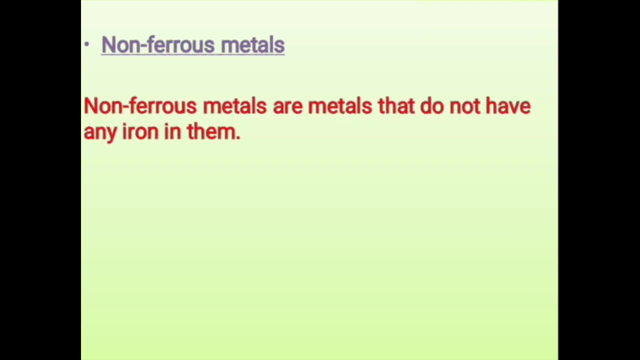 iron and steel. Ferrous are the materials that consist mostly of iron and small amount of other elements. Number second is non-ferrous metals. Non-ferrous metals are the metals that do not have iron in them. They are not attracted by magnet. That's the best point. 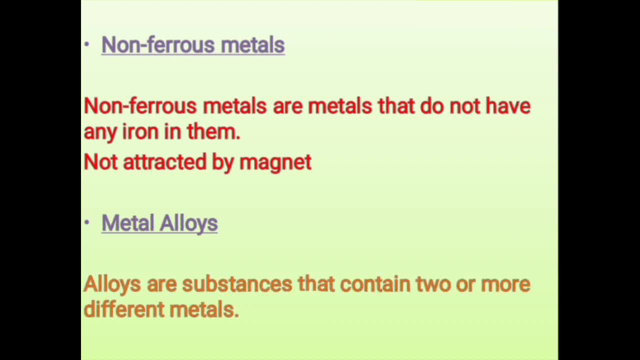 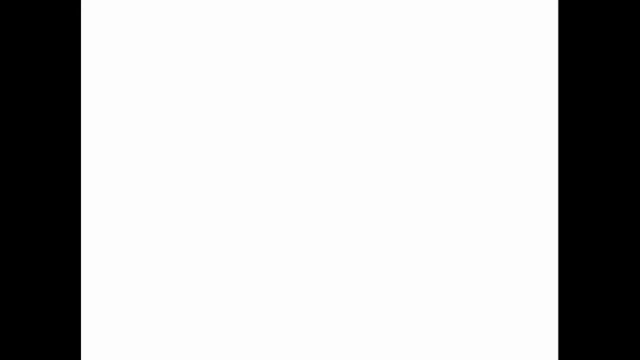 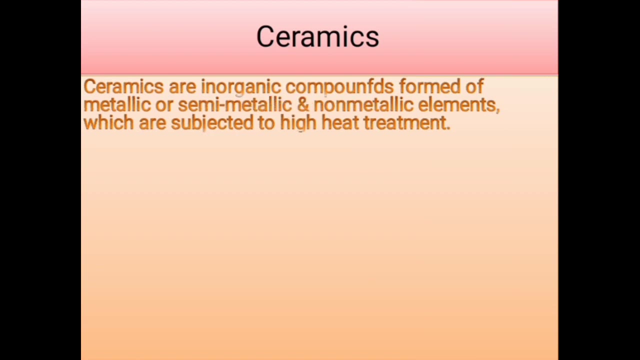 Number third one is metals. Alloys are the substances that contain two or more different metals. Number second classification is Keramics. Keramics are inorganic compounds formed of metallic or semi-metallic and non-metallic elements, which are subjected to high heat. 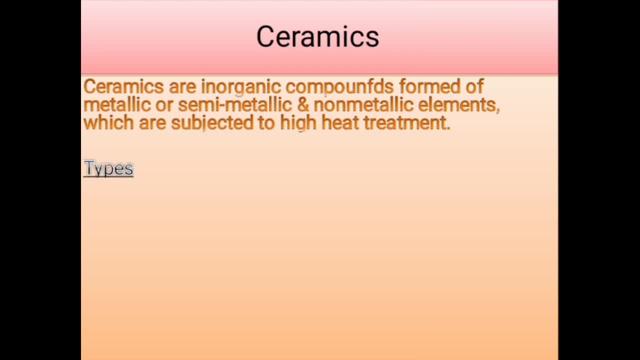 treatment. Number three is the types of Keramics: Structured Keramics that are high temperature load bearing. Number second is refractories: corrosion resistant, insulating. Number third. one is white wares, For example porcelain. Number fifth is glass, Also made up of Keramics, Electrical Keramics, which included capacitors.